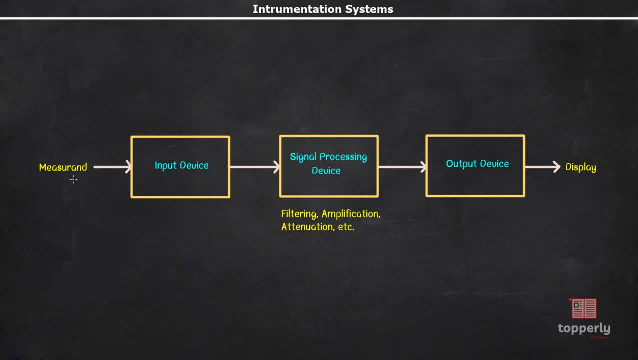 But most often the measurement is a non-electrical quantity. So there is a need to convert this non-electrical quantity to an electrical quantity, And this task is done by a transducer, Specifically speaking an electrical transducer, Because the output of the transducer is electrical. 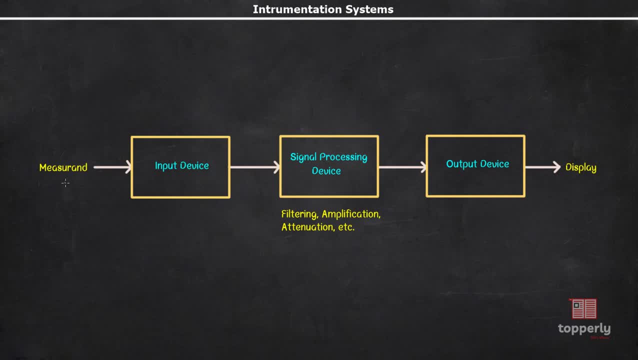 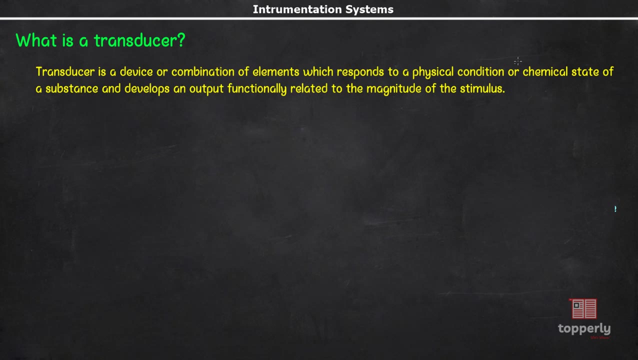 So the transducer will be electrical by nature. Now this output of the transducer can be applied to other components of the measuring instrument. So now comes the question: what is a transducer? A transducer is a device or combination of elements which respond to a physical condition or chemical state of a substance and develops an output functionally related to the magnitude of the stimulus. 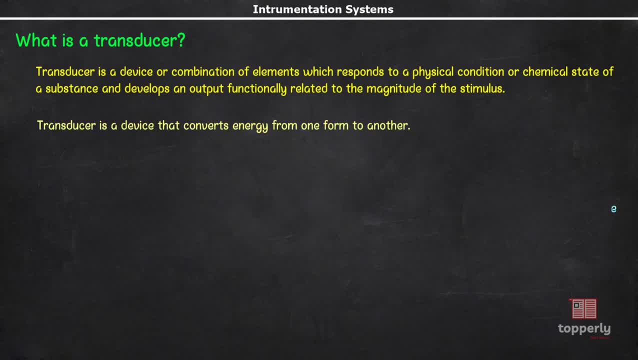 In other words, a transducer is a device that converts energy from one form to another form. Usually it converts a signal in one form of energy to a signal in another, For example optical energy to electrical energy or electrical signal to pressure variation, etc. 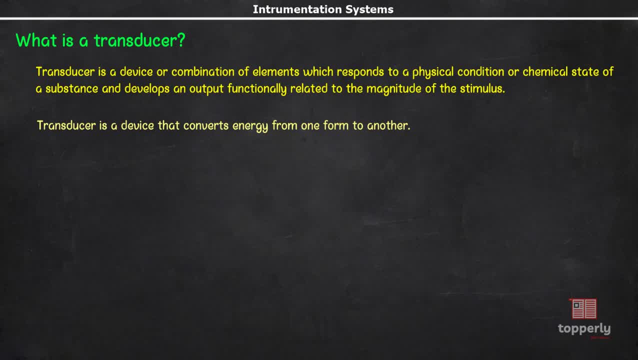 This definition of transducers also reminds us the need for transducers. Suppose our quantity to be measured is in one form and we need to convert it into some other form of energy for the purpose of measurement. Then we can use transducers. 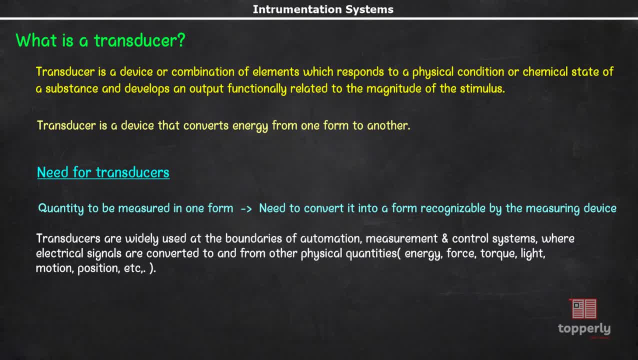 For this reason, transducers are often employed at the boundaries of automation, measurement and control systems, where electrical signals are converted to and from other physical quantities, And this process of converting one form of energy to another is known as transduction. That is transduction. 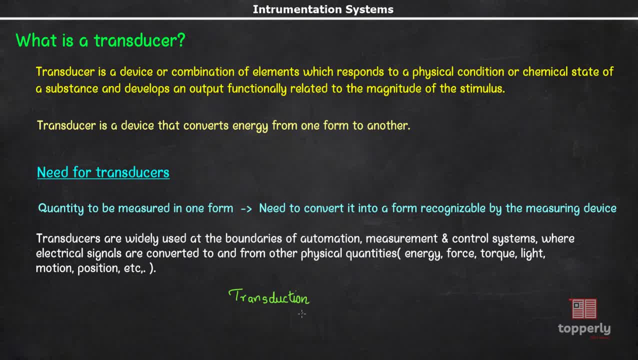 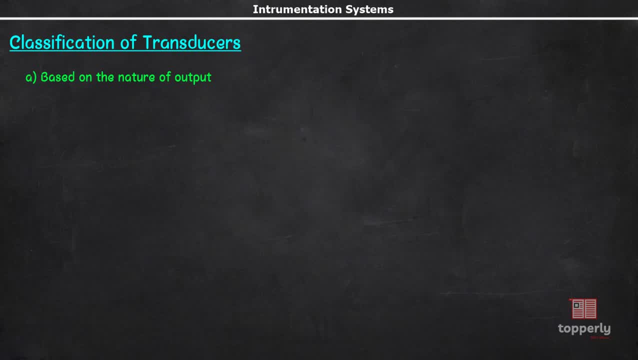 Now going to the classification of transducers. There are mainly two types of transducers based on the nature of output, And they are mechanical transducers and electrical transducers. Transducers that convert physical quantities into mechanical quantities are known as mechanical transducers. 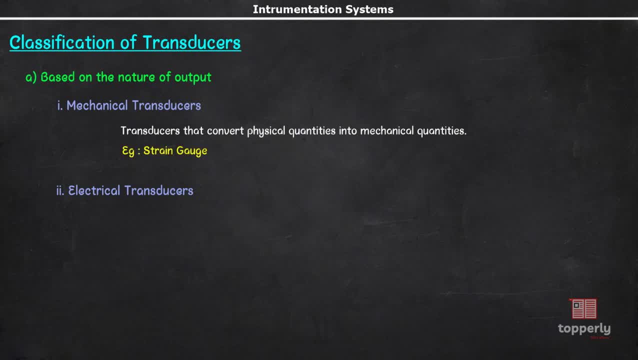 Strain gauge is an example of mechanical transducers. Similarly, transducers that convert physical quantities to electrical quantities are called electrical transducers. An example is a thermocouple that changes temperature differences into small voltages. Now, most often we use these two types of transducers in cascade to obtain the desired signal. 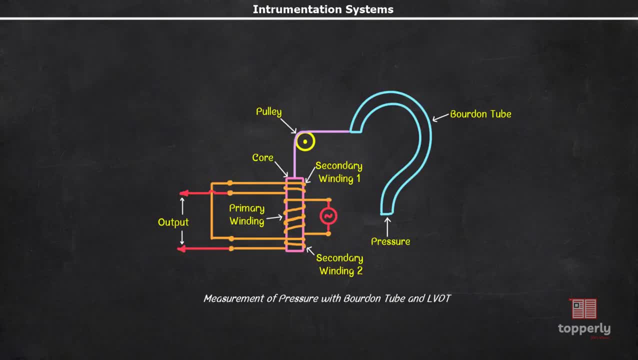 For example, to measure pressure we can use a bourdon tube, But the output of it is displacement. That is, when pressure is applied, the tip of the bourdon tube gets displaced by some amount. However, this displacement cannot be fed to a digital instrument. 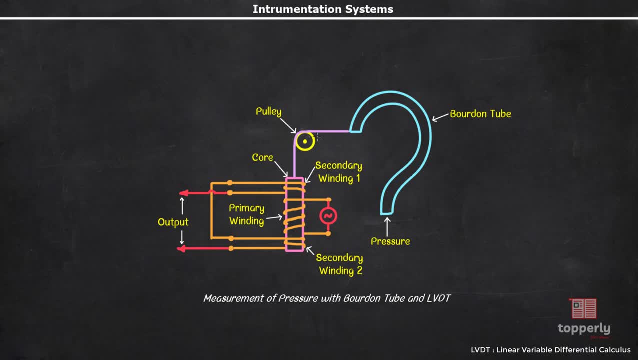 So what we do is, using a pulley and string system. we transfer this displacement to the core of a LVDT. So whenever there is displacement at the tip of bourdon tube, the amount of core inside the winding will be different. 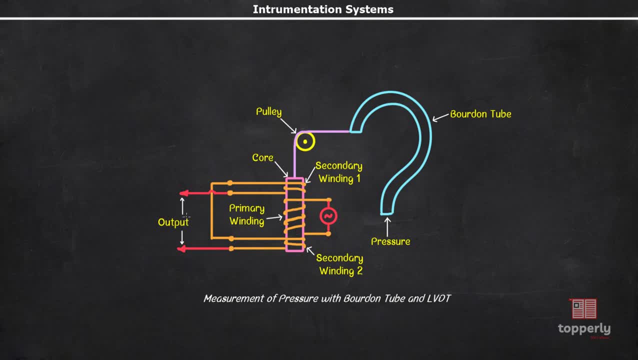 And, as a result, we get an output voltage as a function of the input pressure. And since this output is electrical in nature, it can be fed to a digital instrument. So in this case, you can see that the sensing of physical quantity is done by this block. 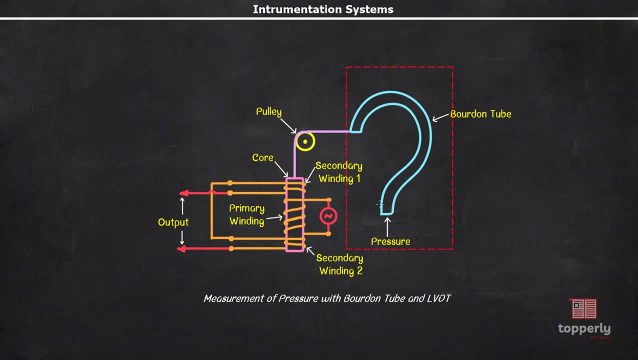 So this element, which is directly coupled to the system under study, is known as the primary transducer. That is, primary transducer, or sensing element or detector element. Now this second block, that is, this block which transforms the output of sensing element, is called a transduction element. 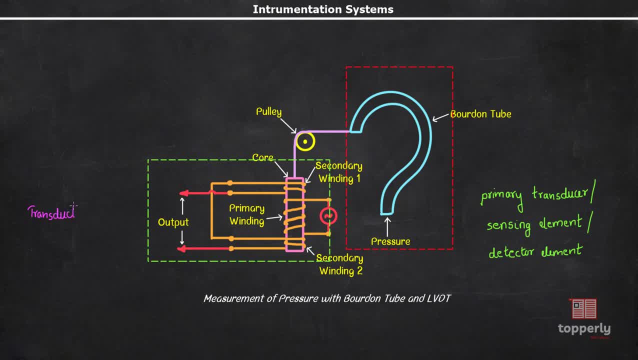 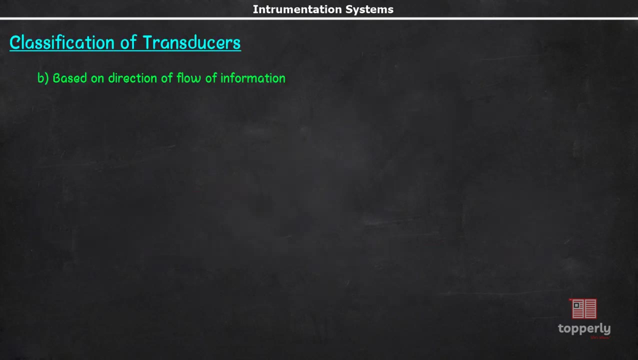 That is, transduction element or secondary transducer. Okay, moving on to the next type of classification, Transducers can also be categorized based on the direction of flow of information. The first class is a sensor. A sensor is a transducer that receives and responds to a signal or a stimulus from a physical system. 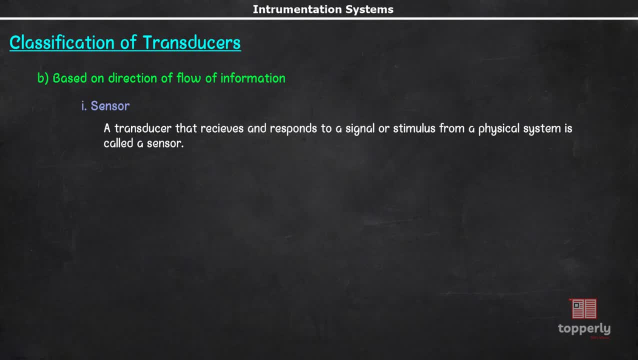 This sensor then produces a signal, which represents the information about the system. An example of a sensor is a thermometer. Now coming to the second class, an actuator. An actuator is a device that is responsible for moving or controlling a mechanism or system. 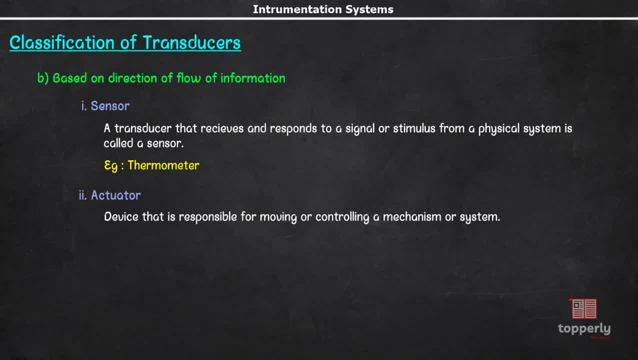 In other words, an actuator is a mechanism by which a control system acts upon an environment. An electric motor can be considered as an actuator, as it converts electrical energy into mechanical energy. Lastly, we have bidirectional transducers. These are transducers that can convert physical phenomena into electrical signals. 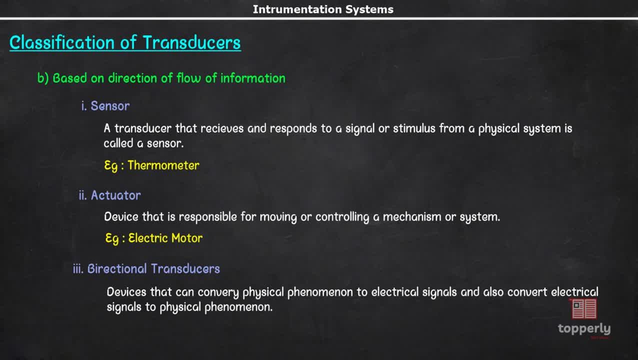 and also convert electrical signals to physical phenomena. An example is an antenna which can convert radio waves into electrical signals and can also translate an electrical signal from a transmitter to radio waves. Now this sensor can again be categorized into two, That is, passive sensors and active sensors. 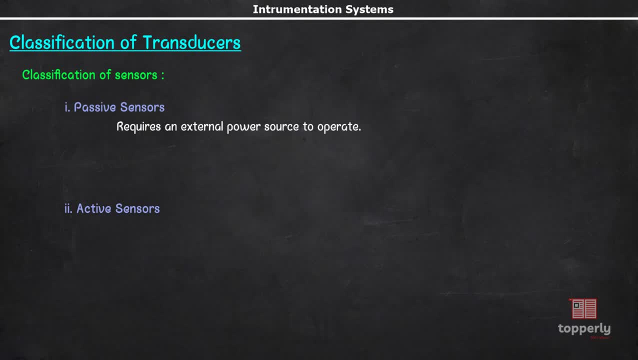 Passive sensors require an external power source to operate, And this external power source is called an excitation signal. We need this external power source because we are actually measuring the power consumed by the sensor in the process of measurement. For example, consider the case of a thermistor. 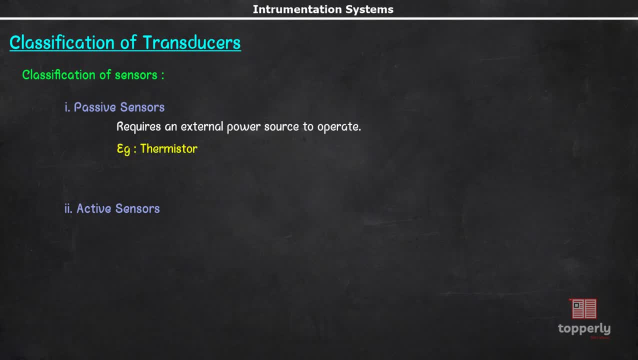 For those who don't know, a thermistor is a type of resistor whose resistance is dependent on temperature. So basically we can sense temperature by measuring its resistance. But for the measurement of resistance we need to pass an electric current through it, as the thermistor does not produce an electric signal on its own. 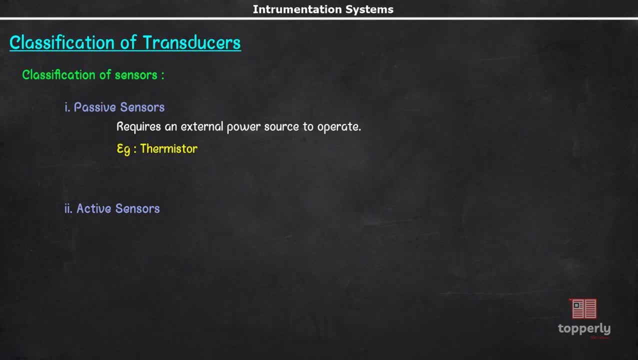 Therefore, you can see that the thermistor depends on external source of electrical power for measurement, So we classify it as a passive sensor. Active sensors, on the other hand, generate an electric current in response to an external stimulus, which serves as the output, without needing an additional energy source. 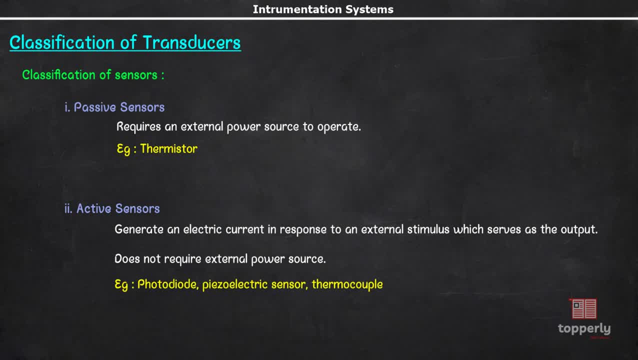 Such examples are photodiode, piezoelectric sensors, thermocouple, etc. Now we will learn another way to classify transducers, which is based on their principle of operation. The first class is electrical transducers, And these are again subdivided into many classes. 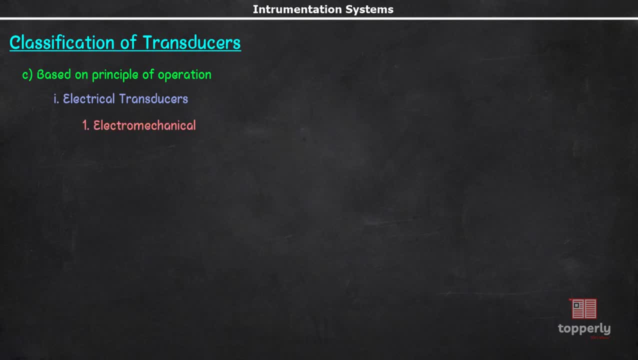 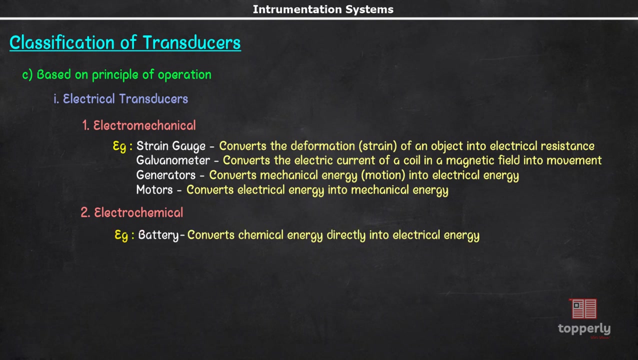 The first one is electromechanical. Some examples of electromechanical transducers are strain gauge, galvanometer, generators and motors. Now the next subclass is electrochemicals, Which includes battery, fuel cell, pH probe, etc. The next subclass is electroacoustic, electromagnetic. 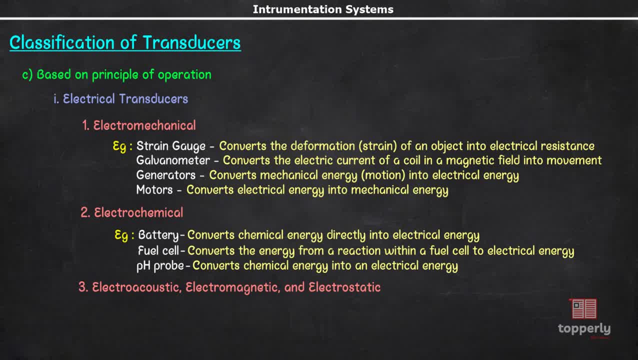 or electrostatic transducers. Example for electroacoustic is loudspeaker, Example for electromagnetic is generator, And for electrostatic an example is Van de Graaff's generator. So these are the three subclasses of electrical transducers. Now the next class of transducers based on operation is: 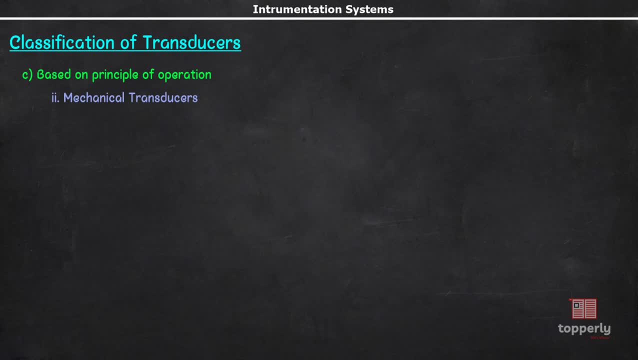 mechanical transducers. Examples of mechanical transducers are barometer, gas flow meter, accelerometer, etc. Then we have thermal transducers, For example a bimetallic strip which directly converts thermal energy into motion. Some other examples are thermometer, calorimeter, etc. 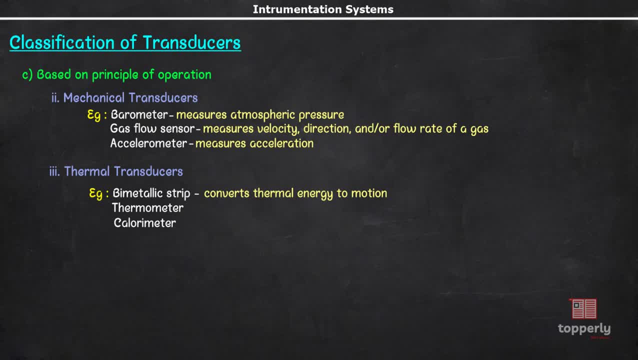 Another class of transducers based on the principle of operation is the radiation type, which includes the photoelectric transducers. Examples are light bulb, photodiode, etc. Again, some other ways to classify transducers are based on the quantity they measure, whether they are analog or digital. 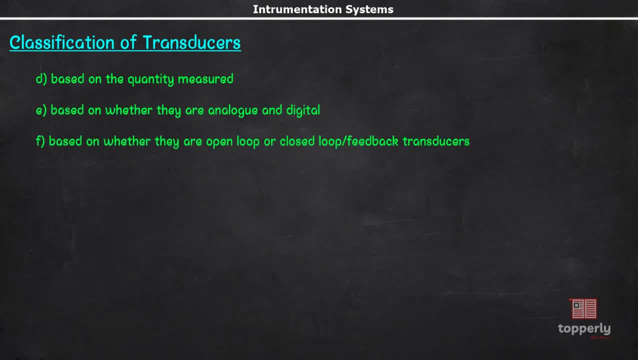 or whether they are open loop or closed loop, feedback transducers, etc. Since these classifications are self-explanatory, I am not discussing it further Now. there are two terminologies that comes under the topic of transducers which you should be familiar with. 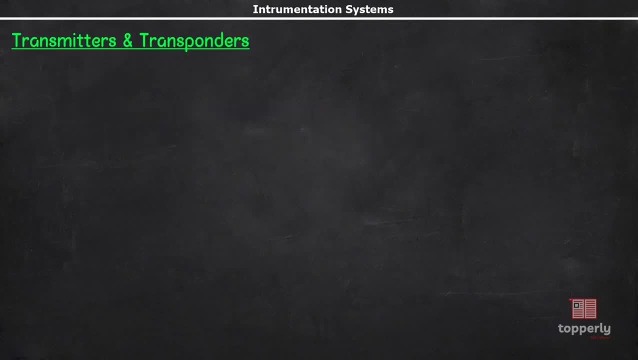 They are transmitters and transporters. Transmitters are transducers that convert the machine into a proportionate signal suitable for transmission over a pair of wires or by means of pneumatic lines. Meanwhile, transporters are transducers, which automatically releases an output signal. 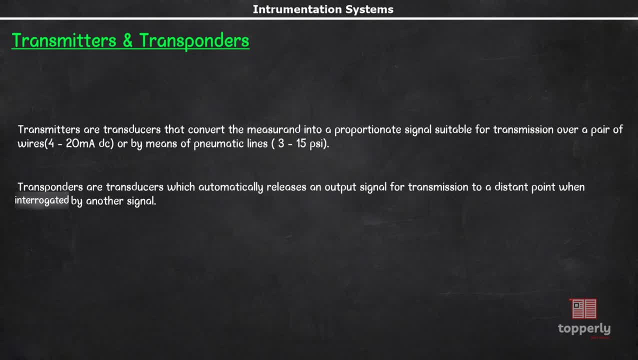 for transmission to a distant point when interrogated by another signal. An example is a RFID device which transmits a coded signal when it receives a request from a monitoring or control point. Coming to our last topic, factors influencing the choice of transducers. 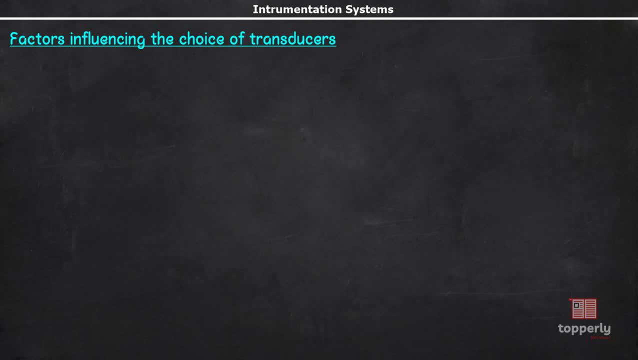 Whenever we are choosing a transducer for a particular application, we have to consider a number of factors into account. Firstly, operating principle. One physical quantity can be measured by several types of transducers. We choose the one with operating principle which best suits our application.